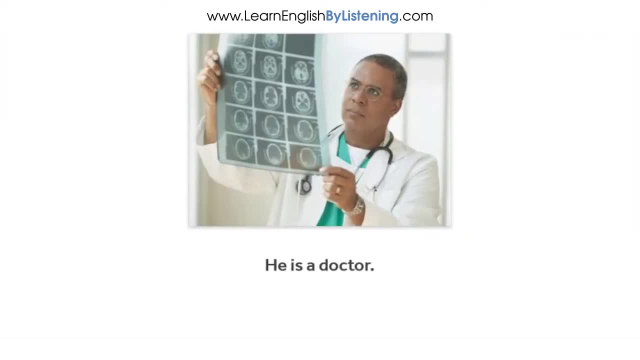 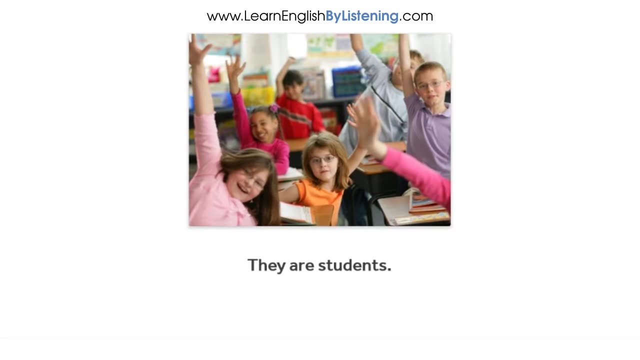 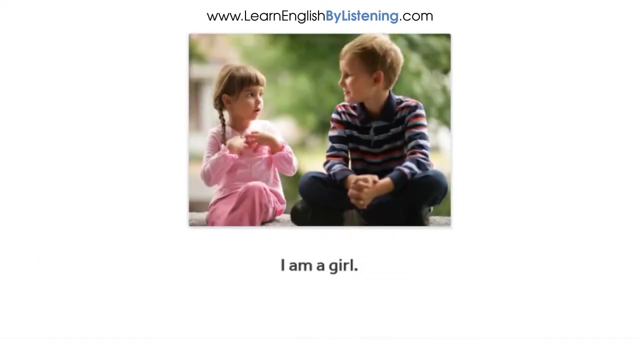 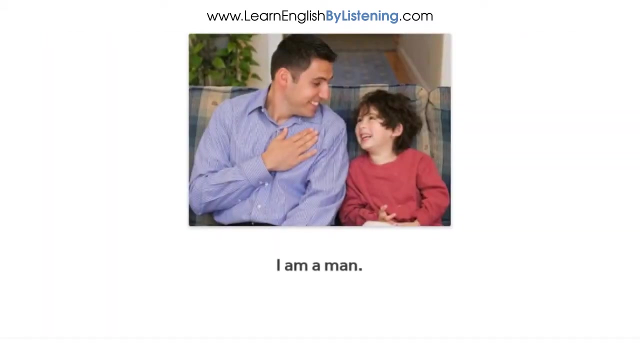 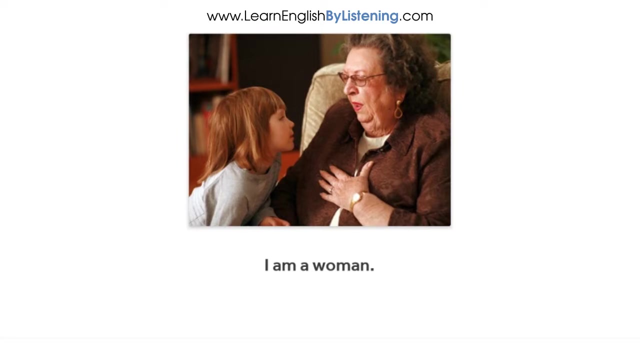 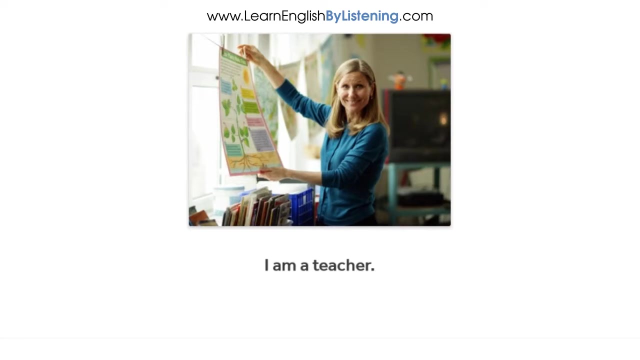 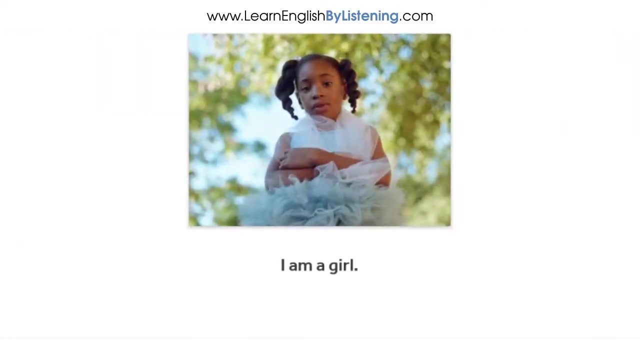 He is a doctor. They are students. I am a boy, I am a girl, I am a man, I am a woman, I am a teacher, We are teachers. I am a girl, I am a girl, I am a boy. 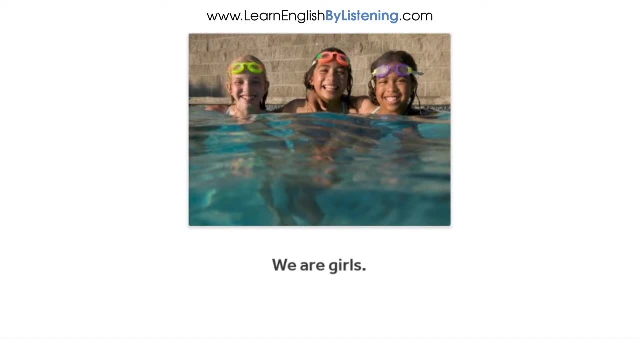 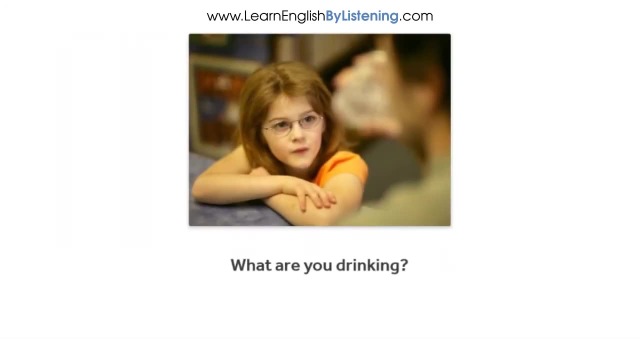 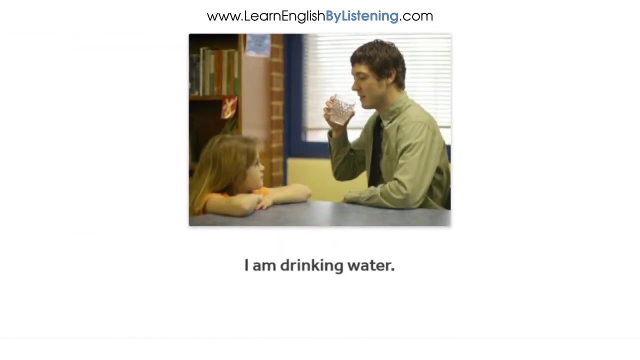 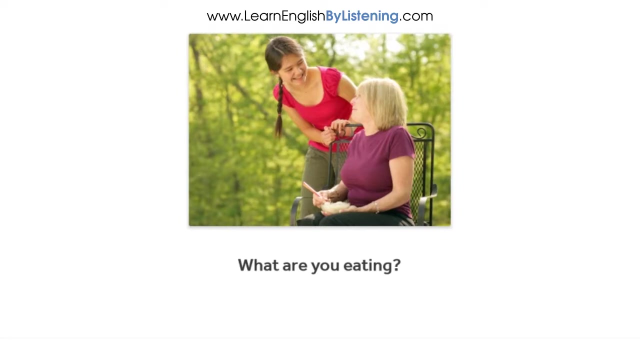 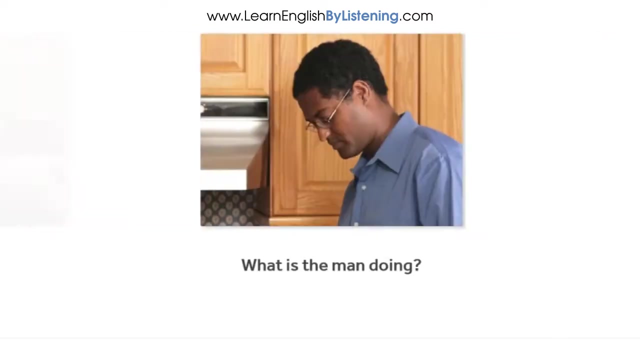 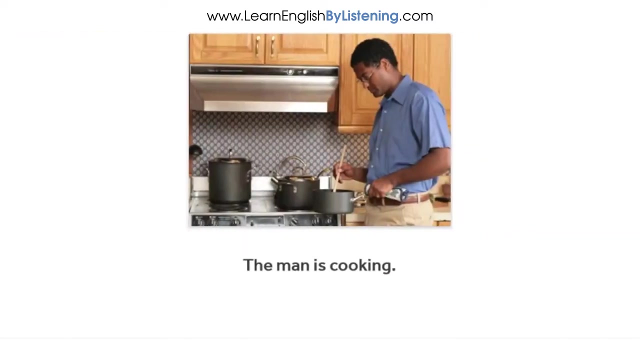 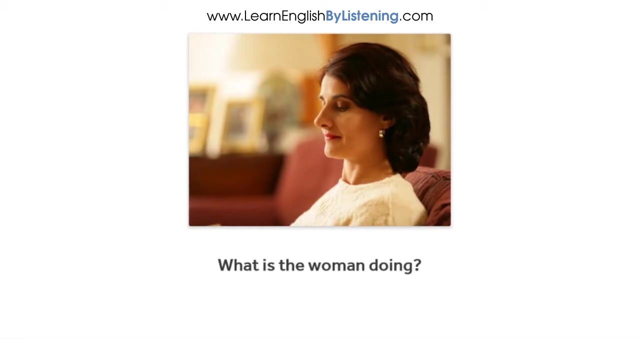 I am a girl, We are girls. What are you drinking? I am drinking water. What are you eating? I am eating rice. What is the man doing? The man is cooking. What is the woman doing? The woman is reading. 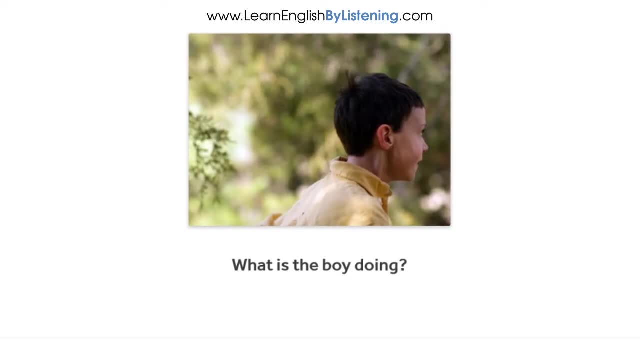 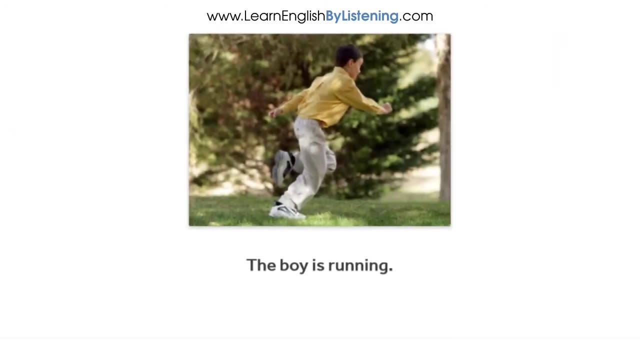 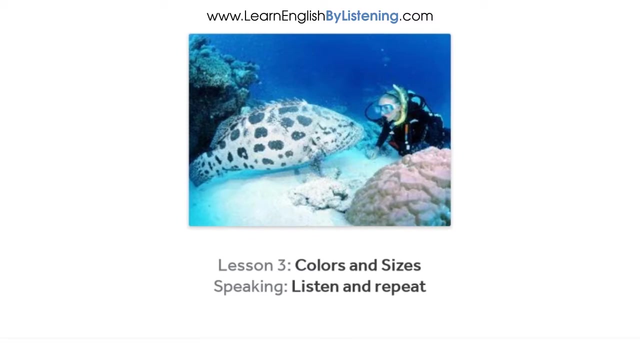 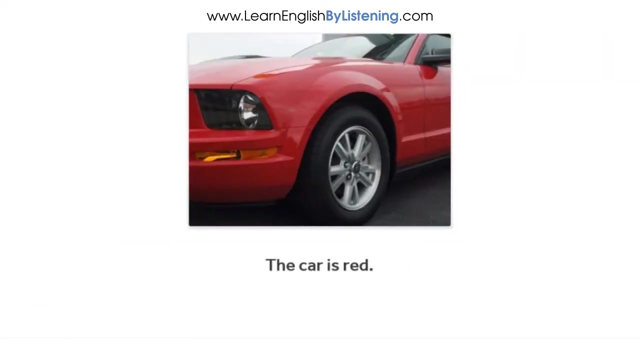 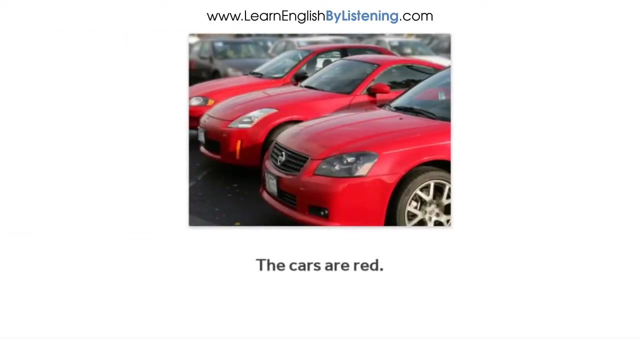 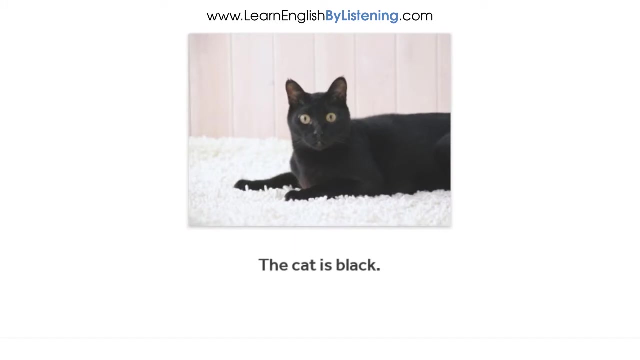 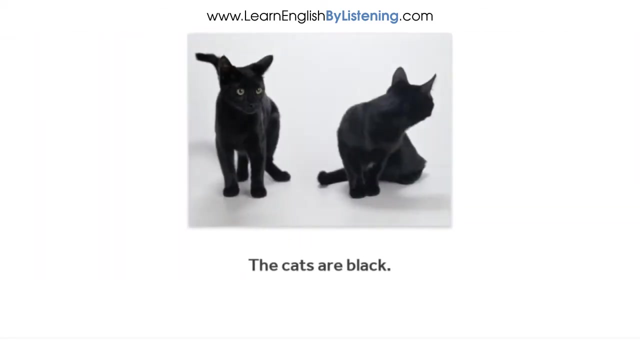 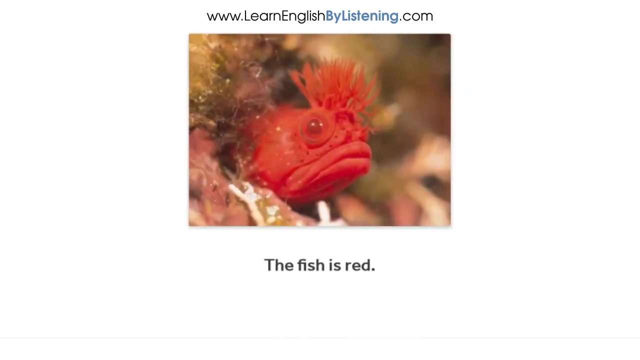 What is the boy doing? The boy is running. Lesson 3. Colors and Sizes- Speaking. Listen and repeat: The car is red. The cars are red. The cat is black. The cats are black. The fish is red, The fish are red. 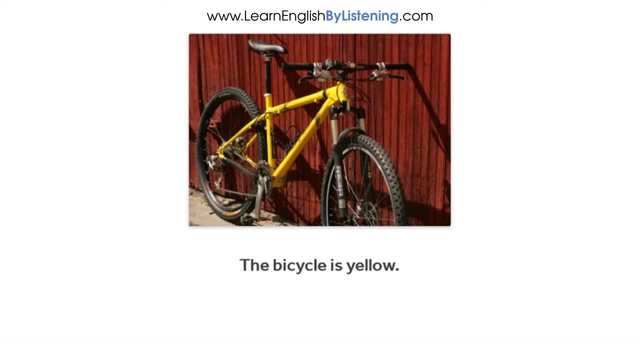 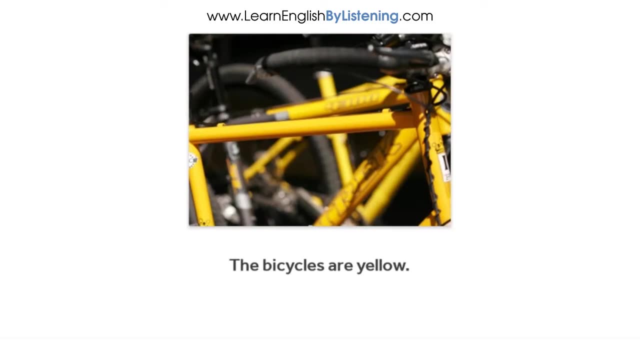 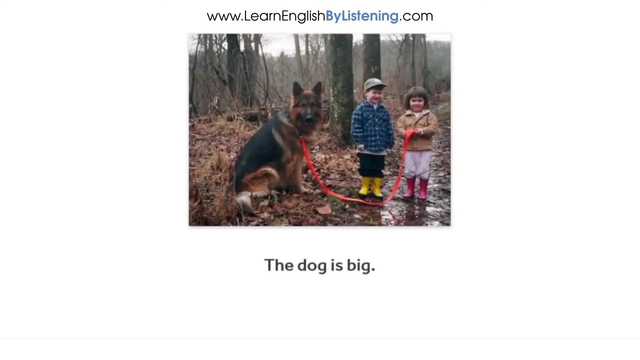 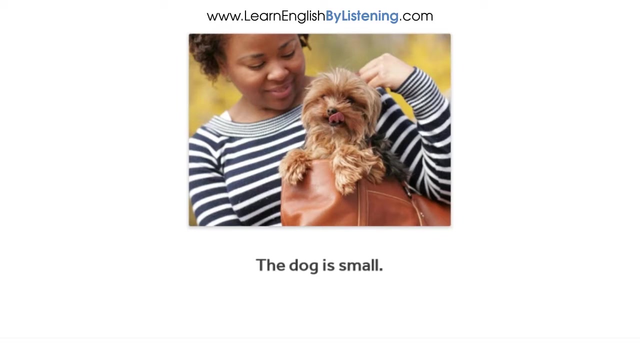 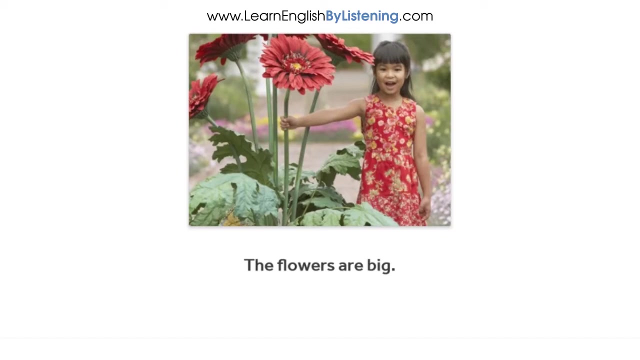 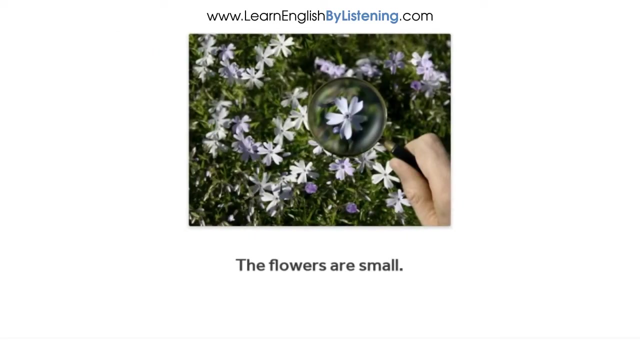 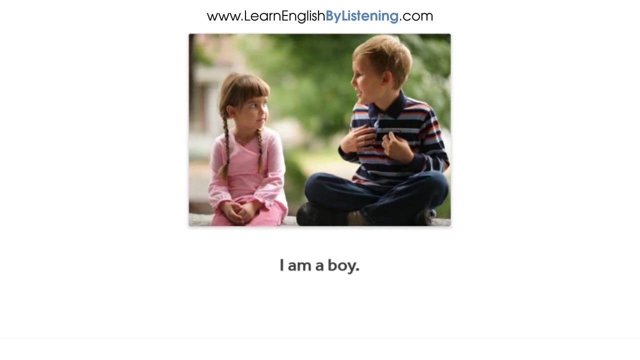 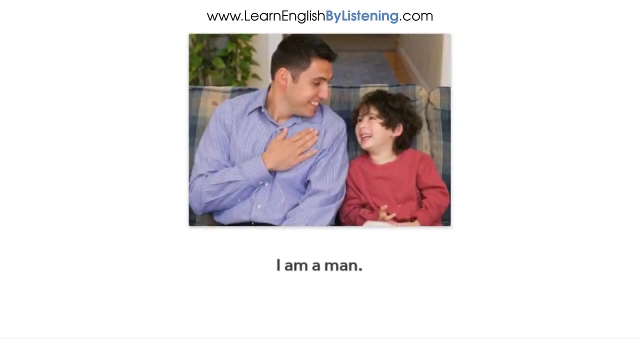 The bicycle is red. The bicycle is yellow, The bicycles are yellow. The dog is big, The dog is small. The flowers are big, The flowers are big, The flowers are small. I am a boy, I am a girl, I am a man. 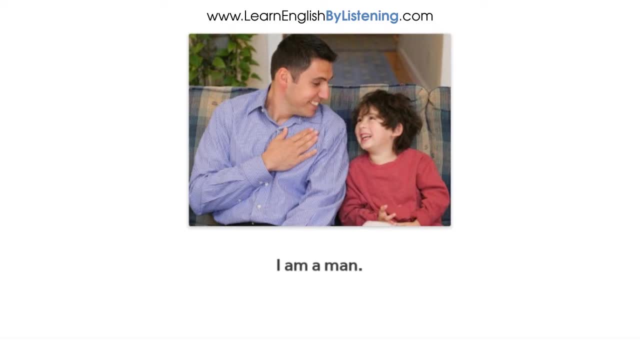 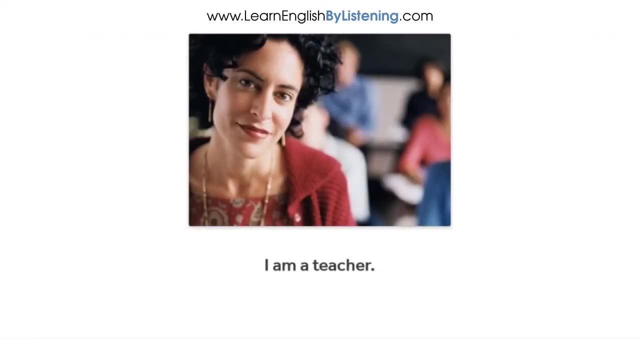 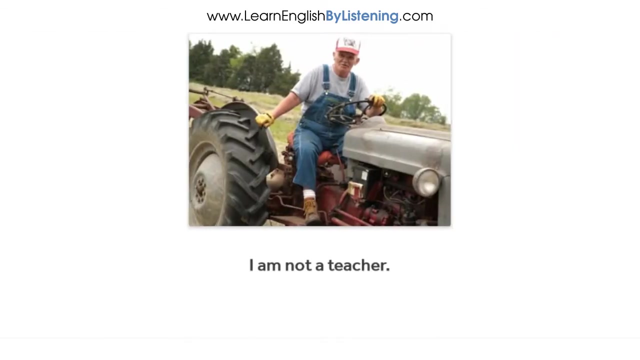 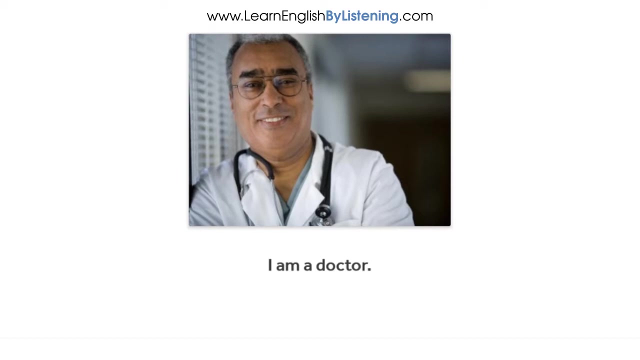 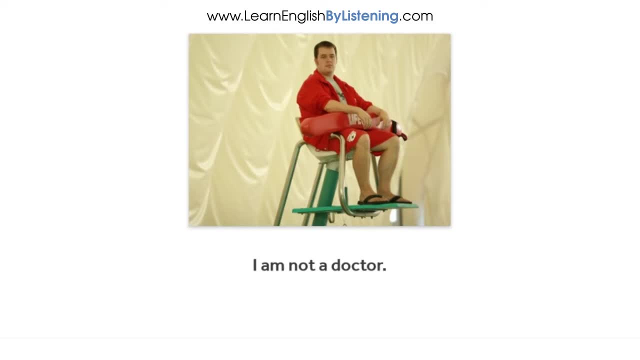 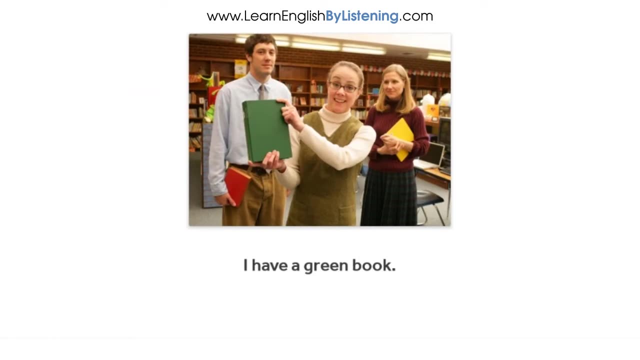 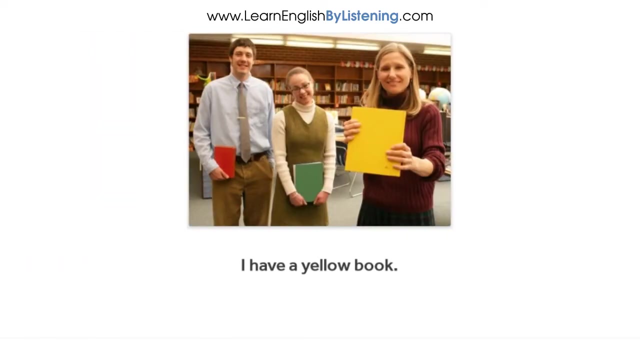 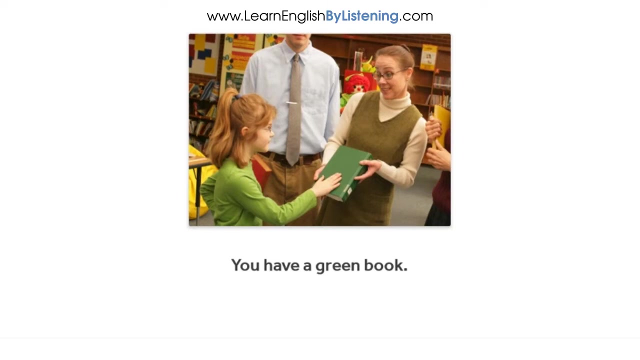 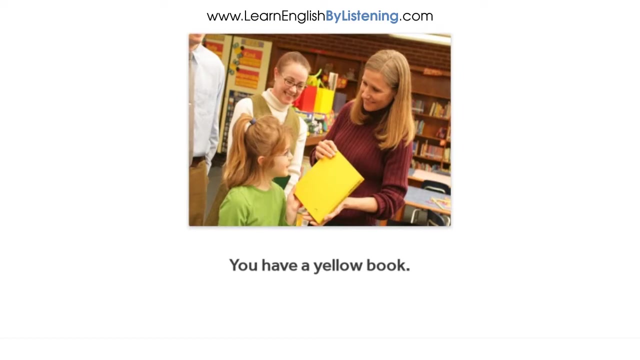 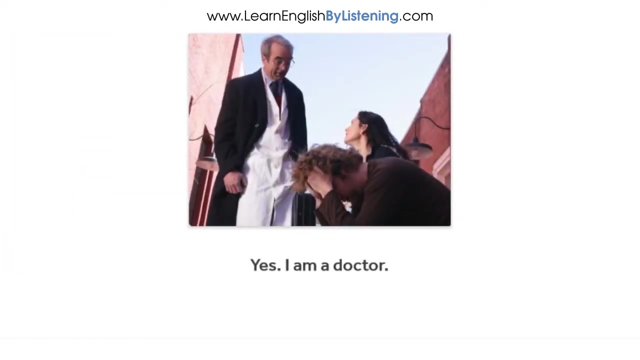 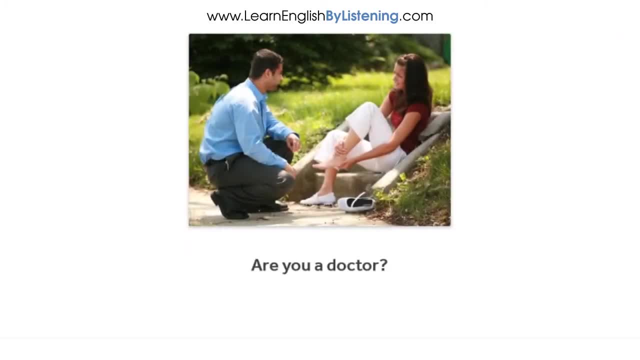 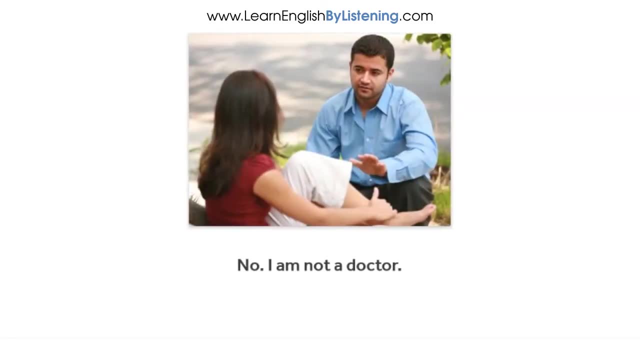 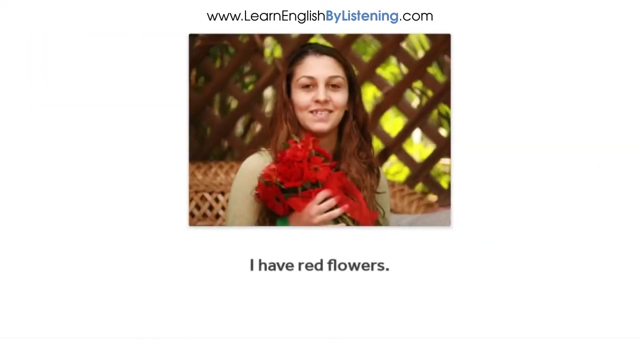 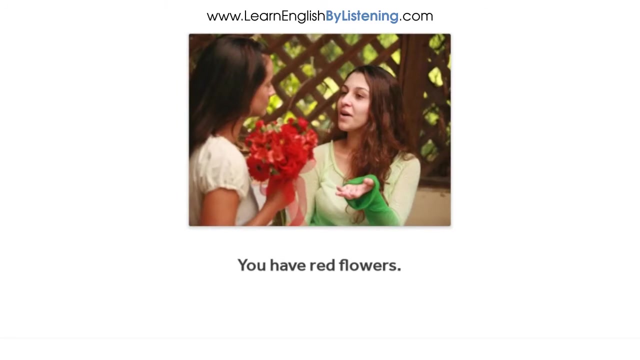 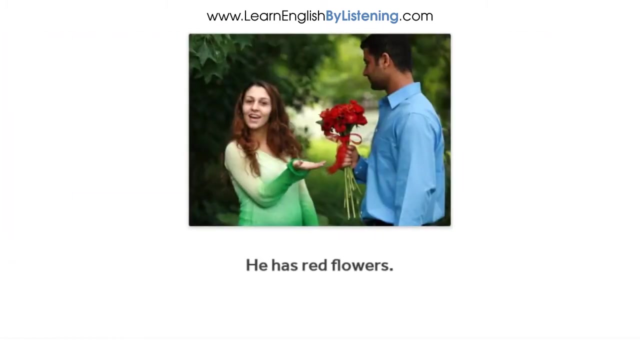 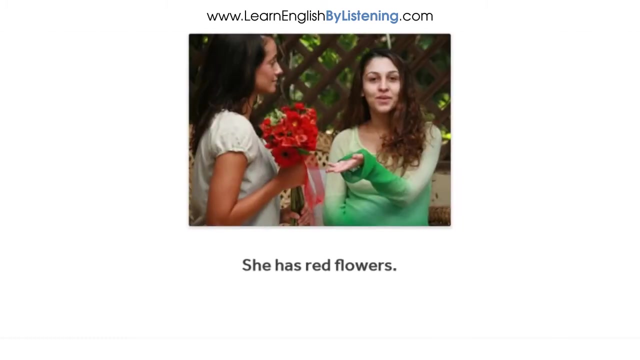 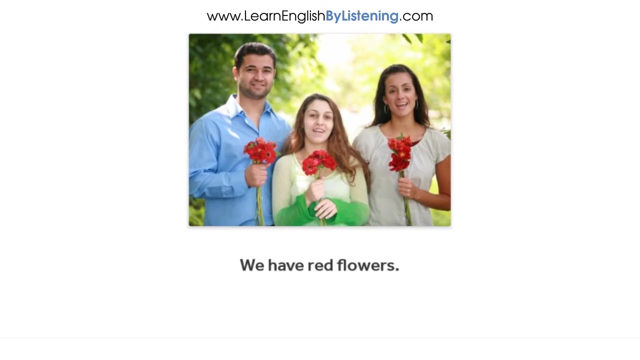 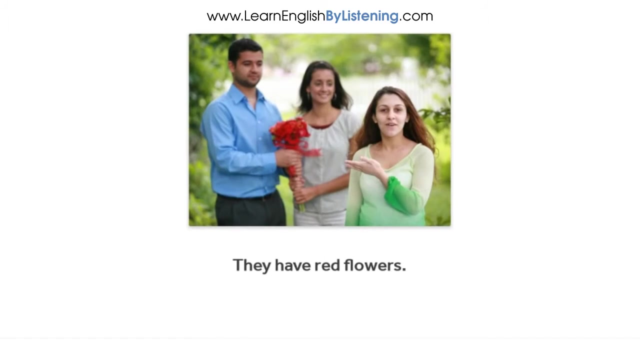 Are you a doctor? No, I am not a doctor. I have red flowers. You have red flowers. You have red flowers. He has red flowers. She has red flowers. We have red flowers. They have red flowers. They have red flowers. 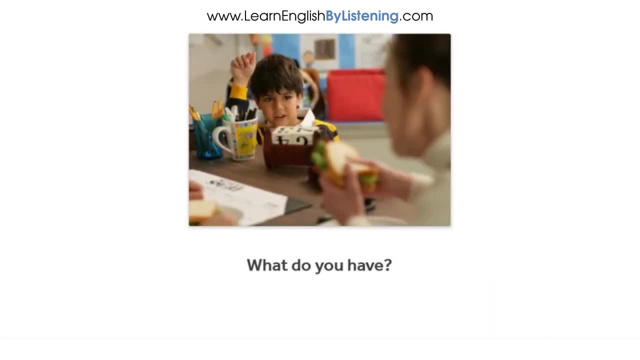 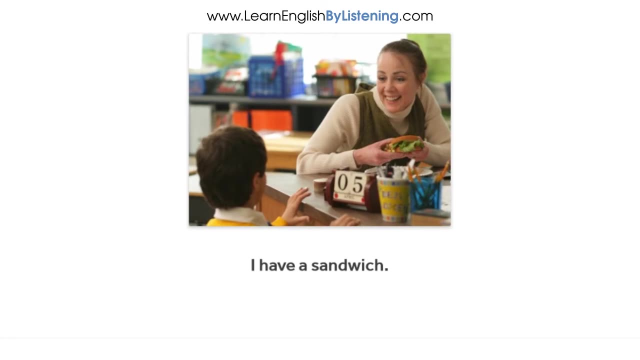 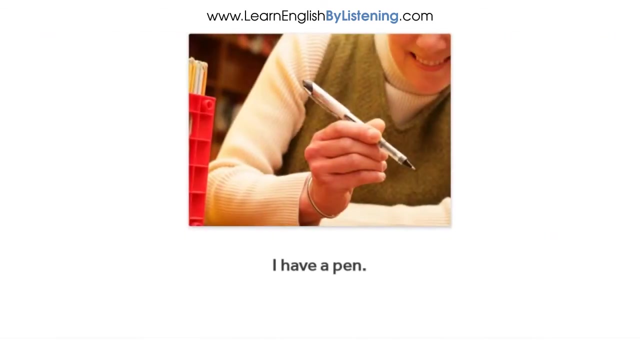 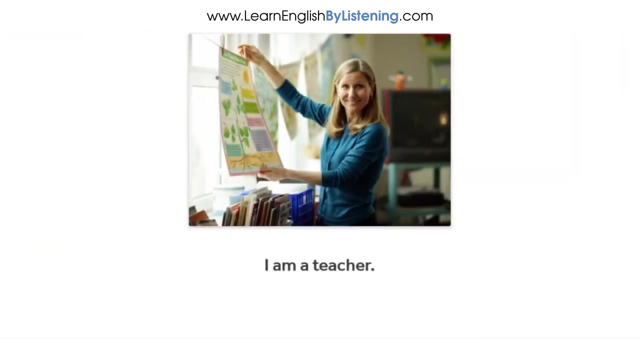 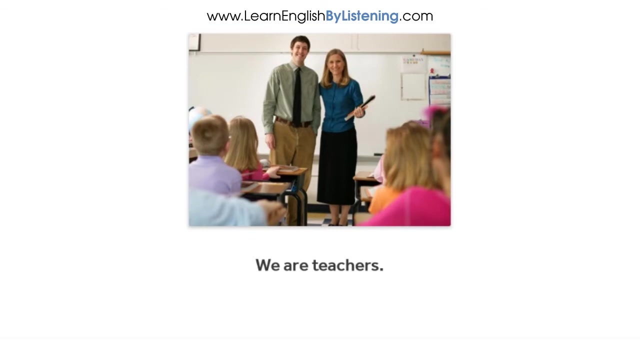 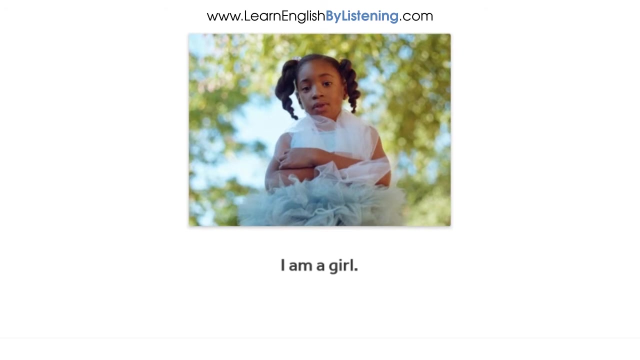 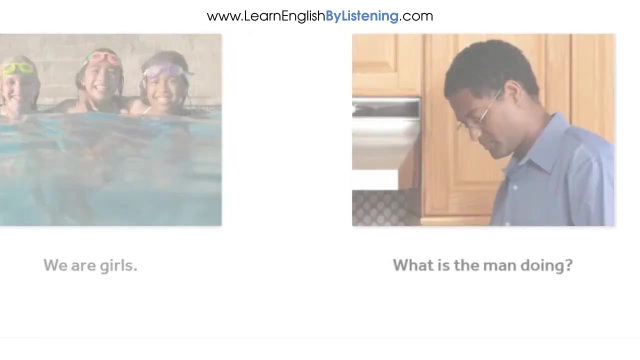 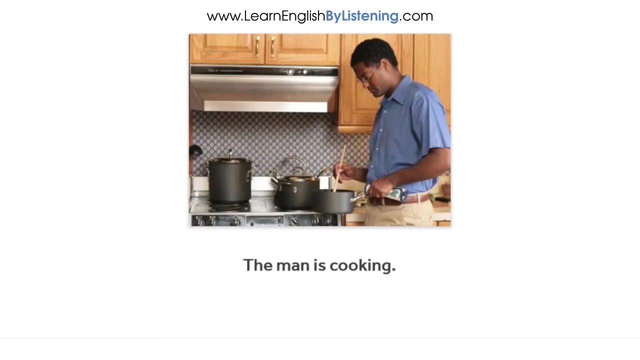 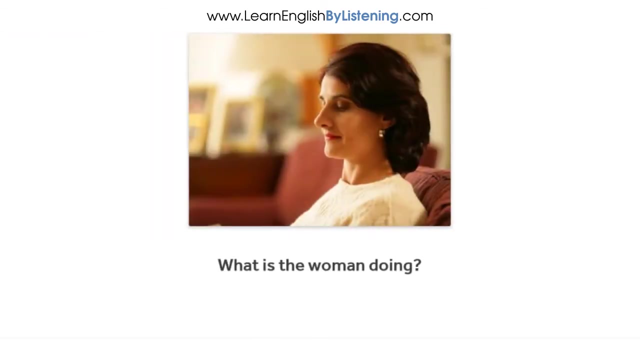 What do you have? I have a sandwich. What do you have? I have a pen. I am a teacher, We are teachers. I am a girl, We are girls. What is the man doing? The man is cooking. What is the woman doing? 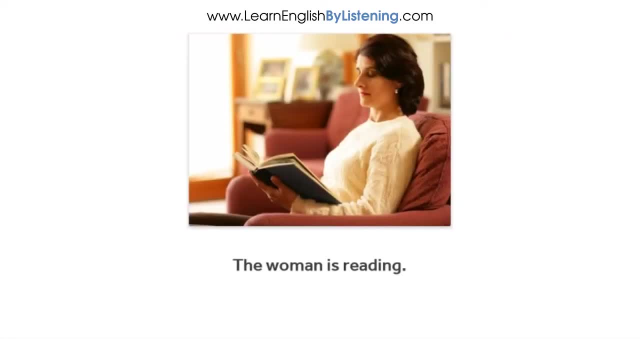 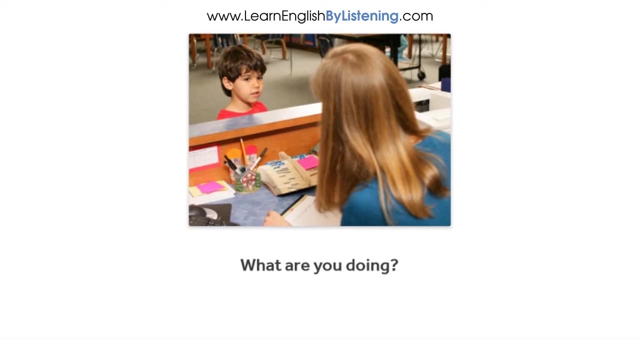 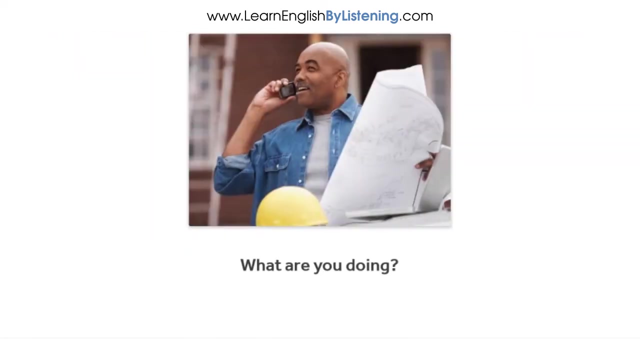 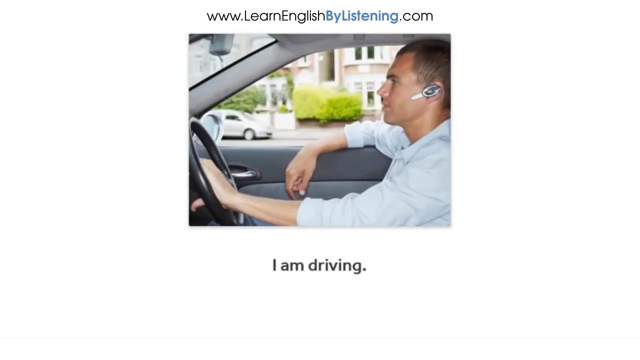 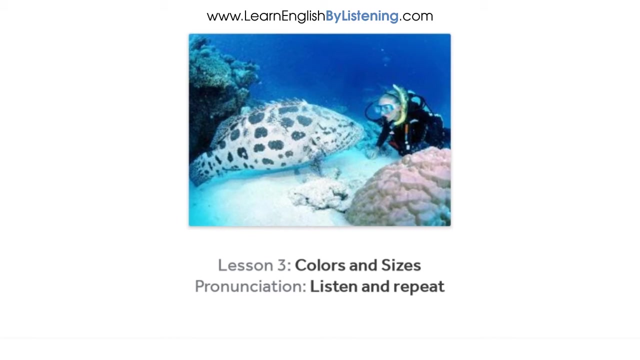 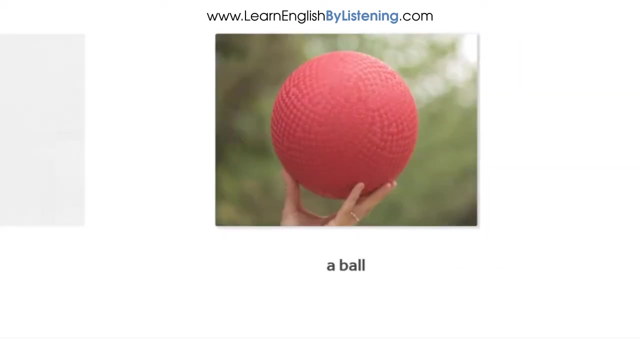 The woman is reading. What are you doing? I am writing. What are you doing? I am driving. What is the man doing? Lesson 3: Colors and Sizes. Listen and repeat, Listen and repeat. black, Black, a ball, a ball. Blue U.